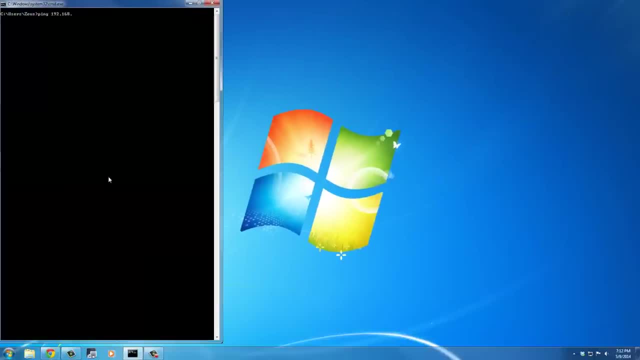 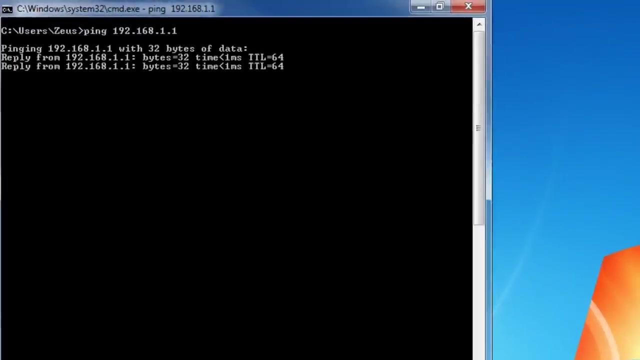 So ping 192.168.1.1.. So what is going to happen here is we are going to send an echo request to the router, and the router is, if it is working, respond with an echo request. So let's press enter And let us analyze these results. So what happened was we pinged the router with 32 bytes of data. So what we sent was we sent a tiny little packet of data that was in 32 bytes of size. 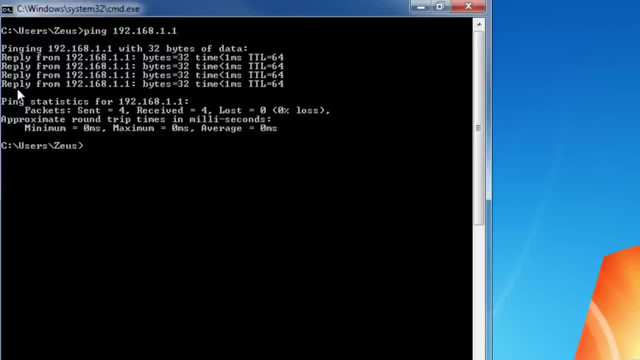 And then I got a reply from the router four times. So this is 1,, 2,, 3, 4.. The ping command by default sends out 432 bytes. And then if you look here, it says the time it took to get a response from the router was less than 1 milliseconds. We sent 32 bytes and the time to live is not that important right now. 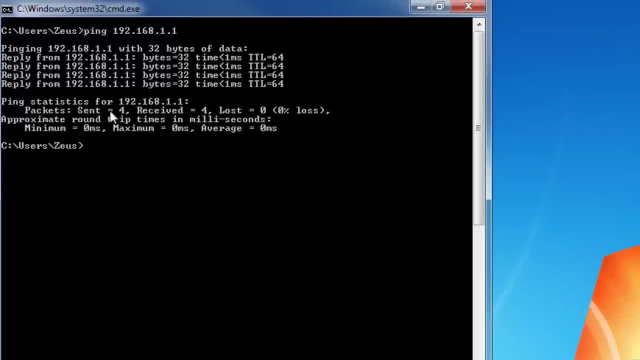 So we can skip that. and then you also get statistics down here. So it says: packets sent 4, packets received 4 and packets lost was 0. So when you see that the packets lost were 0, there is a good sign. That means, of all the packets we sent we got a response right back. So that means our connection is rock solid. So how does this work? as far as network troubleshooting goes, 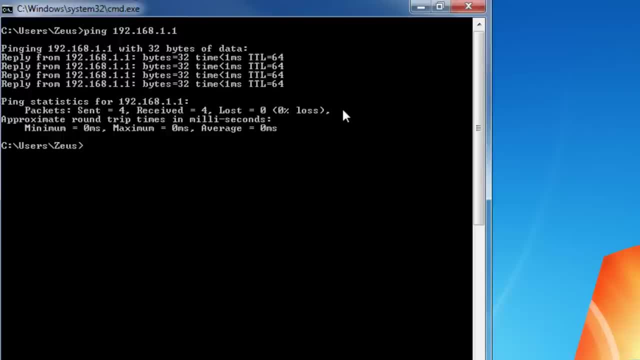 What happens is, as you know, without your router you cannot go to the internet. So if you are unable to go to the internet, your first step should be to ping your router. If the router is working, then you can tell yourself that the router is working. 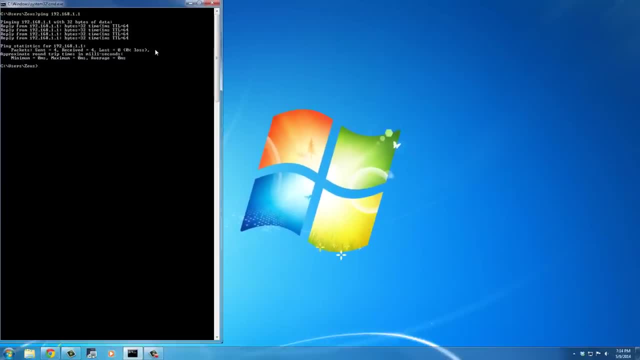 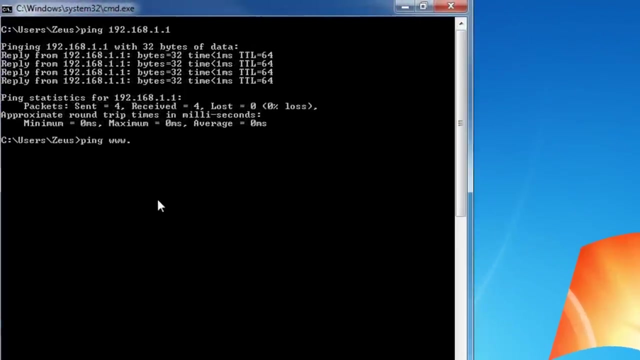 If the router is not the problem. If the router is not working, then you can determine that it is the router that is the problem. Now let's go ahead and ping something beyond your router. Let's ping yahoocom. So let's type in ping and then you can go wwwyahoocom and you can press enter. 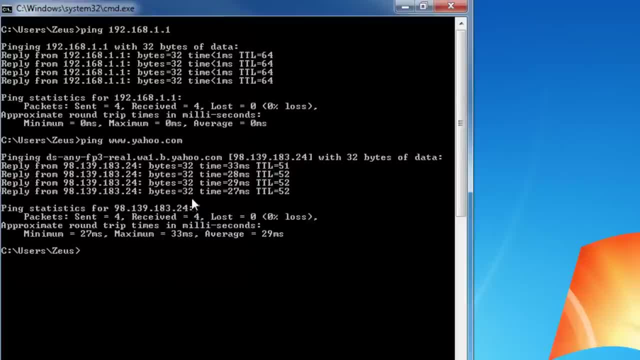 And what I'm going to do is I'm going to analyze the results one more time. So it says pinging. This is the host name, Here is the IP address, The address of yahoo, right here, And we pinged yahoo with 32 bytes of data. So we pinged it four times and every single time we got a response back from yahoocom. 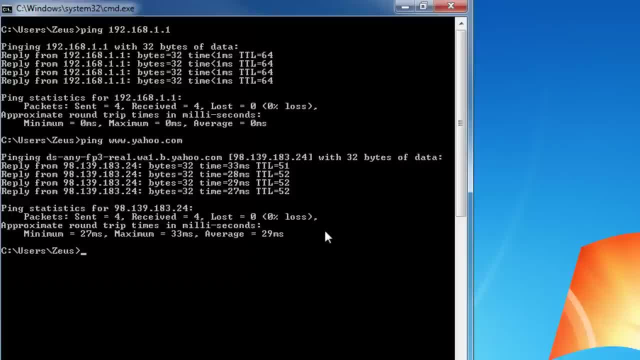 And remember, the response back is the same 32 bytes of data that we sent out. We get it right back, But if you look at each packet here, So let's look at the first packet- The time it took for us to get a response from yahoo was 32.. 33 milliseconds Now if you look at my local router, it was only one millisecond. Now the router is sitting right next to me, But yahoo is probably all the way in another state, So that is why it takes more time to send a packet and receive a response from yahoocom. 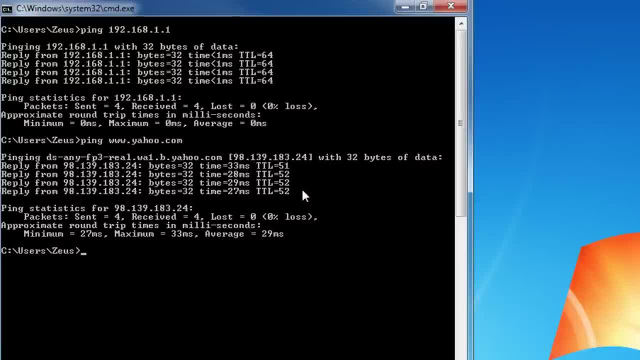 So again, we sent four packets and we got four responses. And if you look down here it says ping statistics for 98.139.183.5.. 24, which is the IP address of yahoo. We sent four packets, We received four packets, We lost zero packets. So what does that mean? 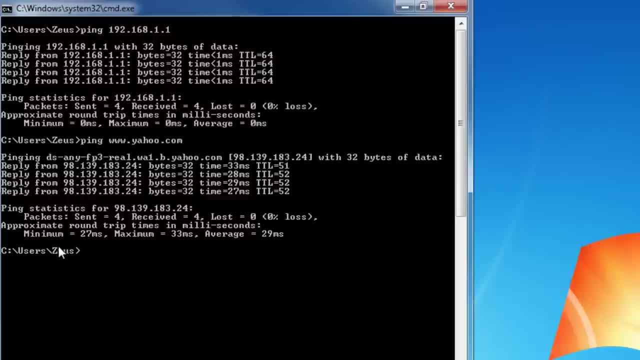 That means the connection is in fact rock solid And if you look down here, The minimum time to get a response from yahoocom was 27 milliseconds, Which is the 4th packet right here. The maximum time to receive a response from yahoocom was 33 milliseconds, Which is the packet over here. 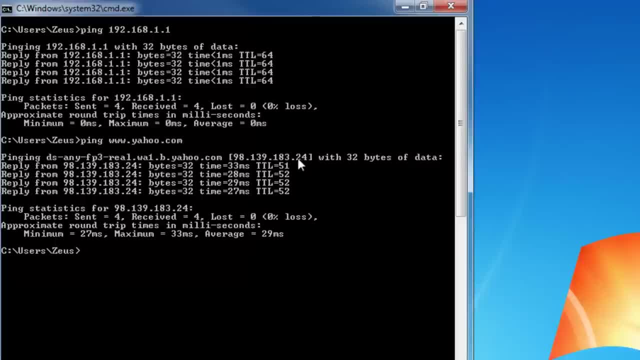 And the average is 24.. nine milliseconds, which is the addition of all these divided by four. now, so the ping command is all about analyzing the packets. you send out a packet, you run the ping command, you send out some packets and you analyze the results for. 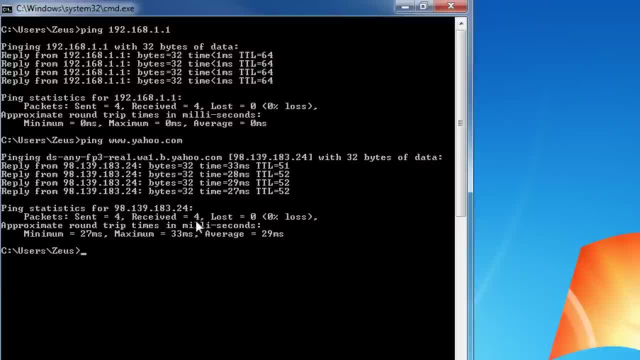 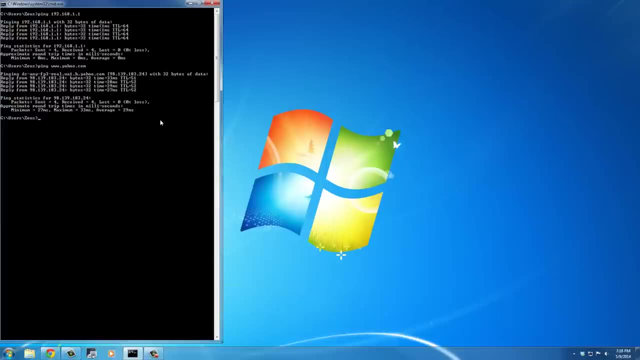 example, if I had sent four packets and I received only one packet back, my lost packet numbers would be three. so that would mean that there's a connection problem somewhere in the line from me to yahoocom. but this is. that is the first step in diagnosing a problem. now, as another example, let's ping something. 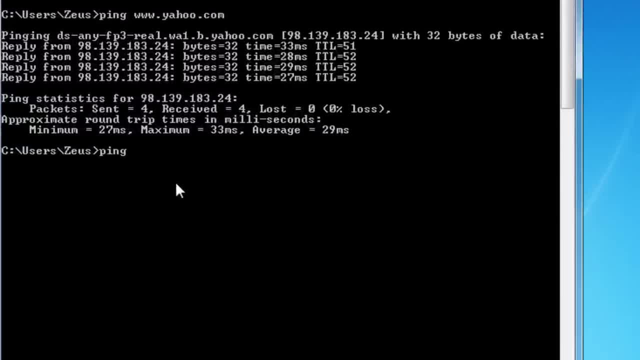 that doesn't exist and see what happens. so let's do ping one nine, two dot. one six eight dot. one dot five thousand. okay, so I know for a fact that that IP address does not exist on my local area network. so if I press ENTER it says ping request could not find host one nine two dot. one six eight dot. 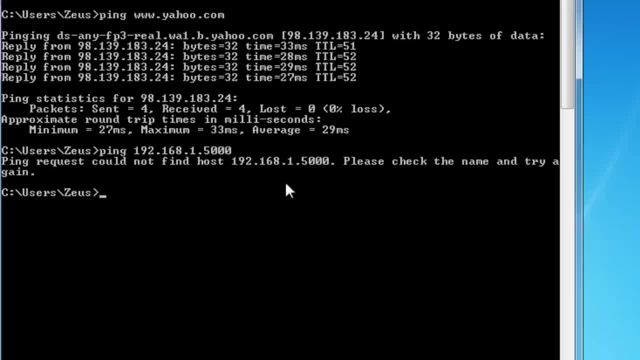 one dot five thousand. please check the name and try again. so let's say that one nine two dot one six. eight dot one dot five thousand was a server on my local area network. I tried to ping it and I did not get a response. so what does that? 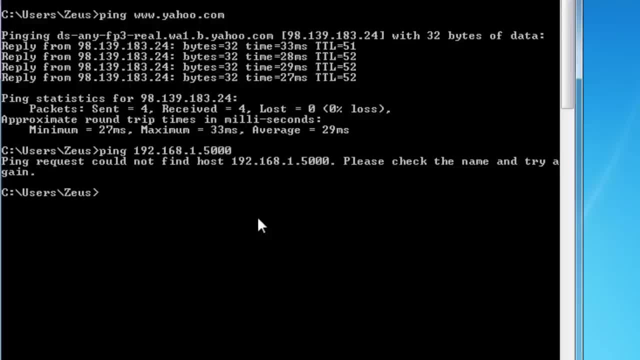 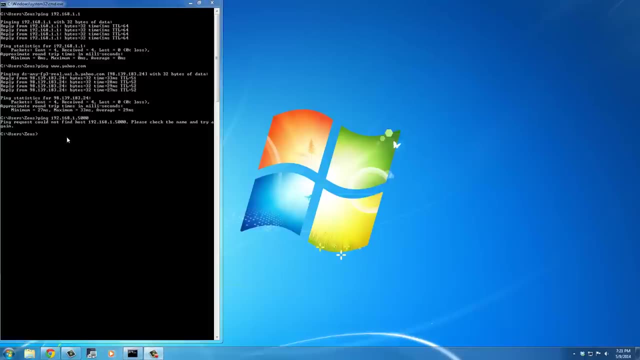 mean? that means it's not working. so I have to go to my server and I would have to configure it to make sure it is working. we check the cables. I would make sure the server is turned on and that is configured properly. okay, all right, so let me just type in CLS, which clears the 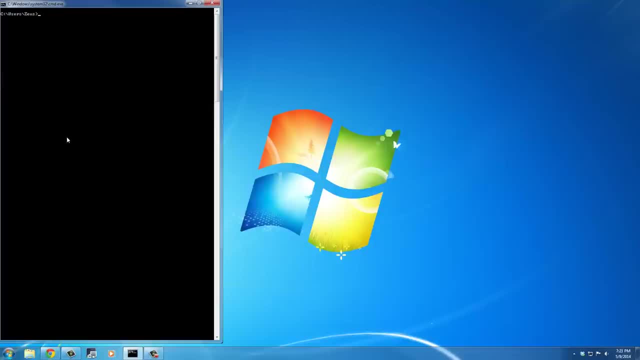 screen and I'm going to show you other things you can do with the ping. so the ping command is a little more advanced than what you just saw. that what you just saw were the basics. you can manipulate the ping command to increase the size of the packet you're sending or maybe increase how many times you want. 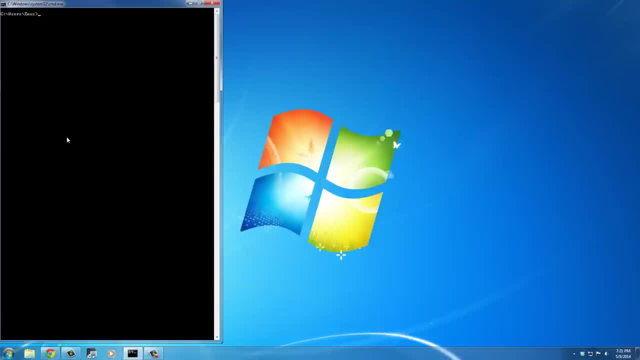 to ping the server, and that's what I'm going to do. so I'm going to go to my server and I'm going to show you how to ping a particular device. so let me show you how that is done. and how you do that is by using parameters right after the. 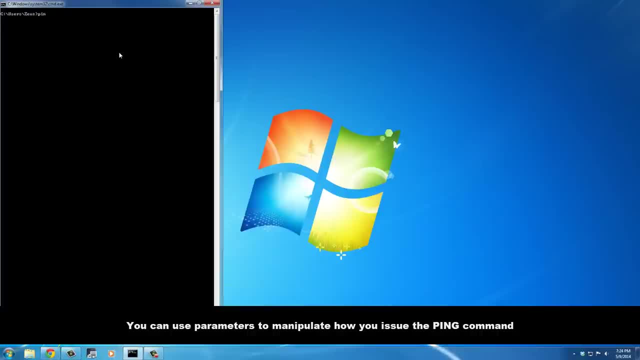 ping command. so I'm going to go over two very important parameters. number one is going to be ping, and then what you do is you type in minus n, okay, and then you put in any number. don't put a big number, put like something like um, let's say. 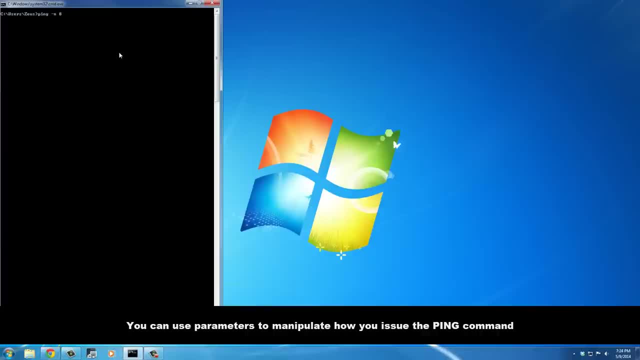 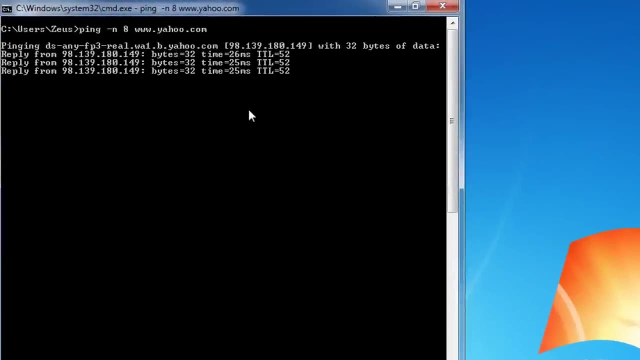 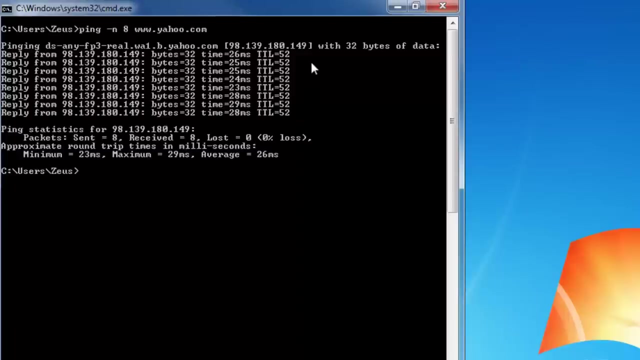 eight, and then let's ping Yahoo eight times. so this is what this parameter is. this parameter does: you can change the number of times you want to send a data packet to yahoocom. so wwwyahoocom and watch what happens now. okay, so instead of sending Yahoo four packets, that we usually do by using the 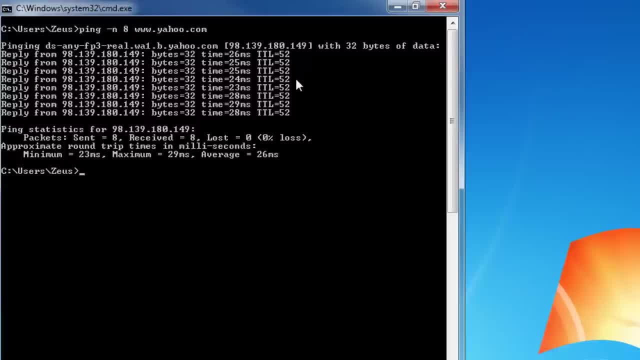 ping command. all by itself we were able to send Yahoo eight packets. okay, so this is one, two, three, four, five, six, seven, eight, and if you look at the bottom here, packet sent eight, received eight, lost zero. so that means again, the connection is rock solid. we did not lose any packets out of eight packets. 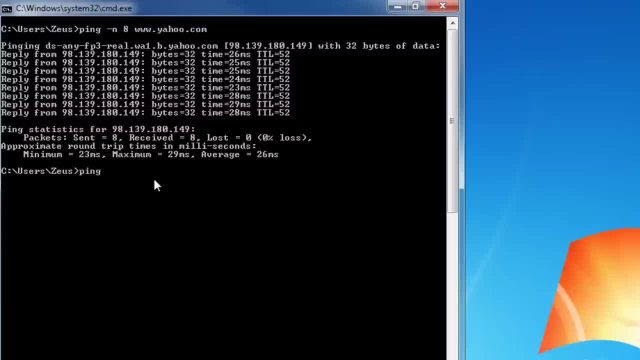 alrighty, let's do one more, let's do ping minus and let's do 10 packets. let's do with Google, this time googlecom. So we are going to use, we're going to say ping, We're going to put this parameter minus n After the parameter. you put in how many packets you want to send And then you type in the destination IP address or the destination address. 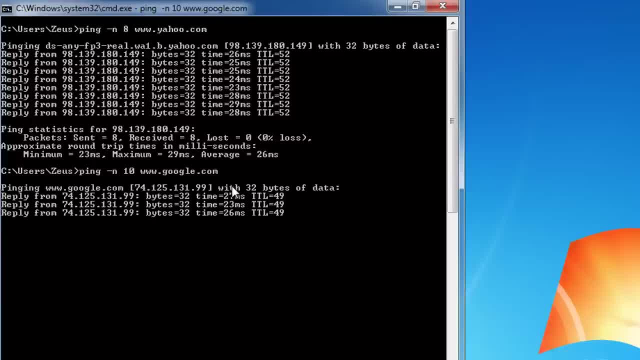 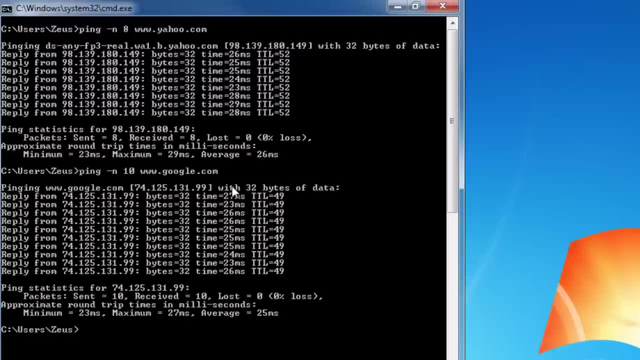 Okay, so press enter 3,, 4,, 5,, 6,, 7,, 8,, 9,, 10.. Again, we sent out 10 packets, If you look at the bottom here. So remember ping statistics for 74.125.131.99.. That is the IP address of the Google server. 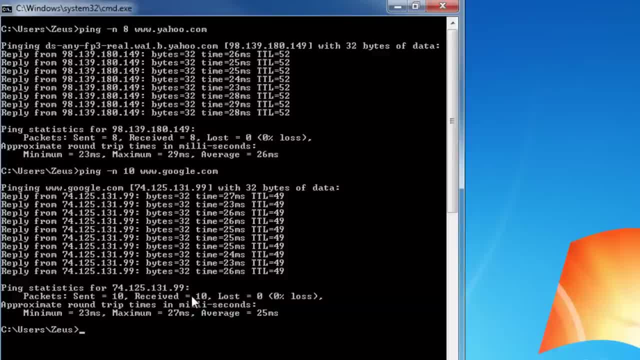 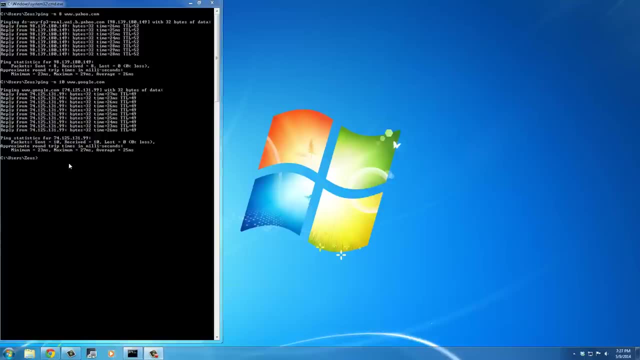 So we sent 10 packets, We received back 10 packets. So we received 10 echo responses from Google And we lost zero packets Again. that means the connection based on these statistics here is rock solid. Okay, so that was the first parameter I want to go over. It's a nice way to extend how many packets you can send, which gives you greater control over trying to diagnose a problem. 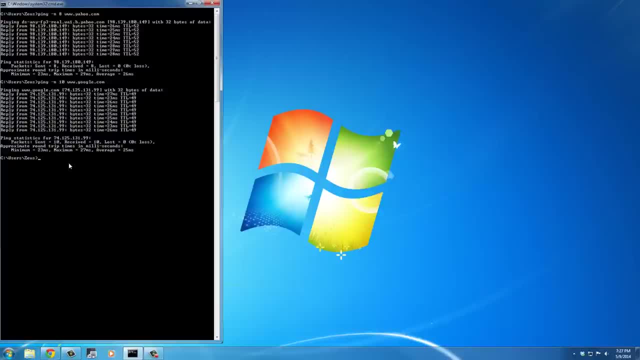 So if you send four packets, that is not a big deal- Anybody can send and receive four packets. But what if you send 100 packets to Google? You're bound to lose a packet or two, which will kind of tell you if your connection is in fact solid or there is some problems here and there. 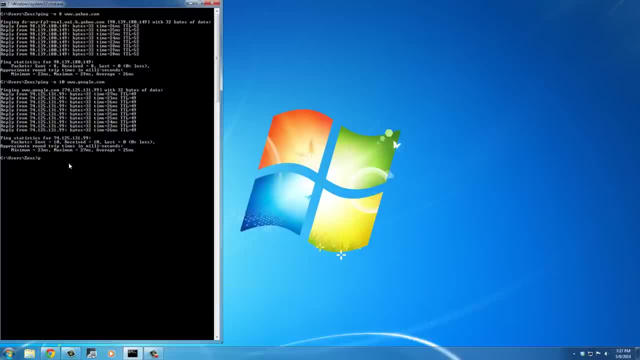 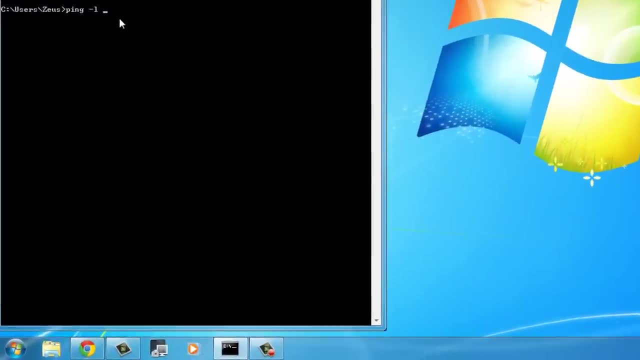 Anyway, let's go to the next parameter. So let's type in ping, And this time I'm going to use minus l, And what this allows me to do is it allows me to designate the size of the packet. So if you look up here, the packets by default are 32 packets. 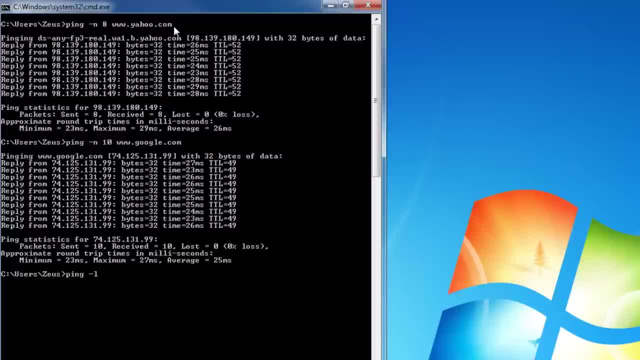 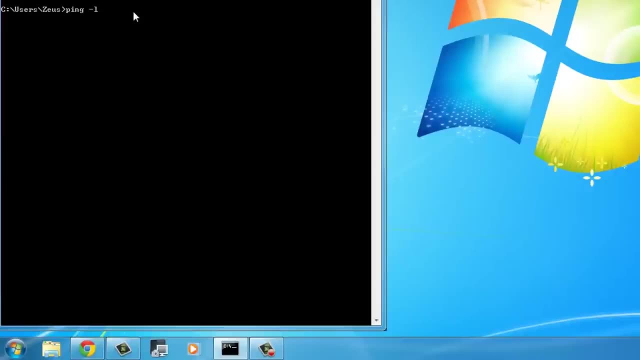 So that's the first ping, And even the ping on the top for Yahoo is 32 bytes. So by default, our packets, our sized 32 bytes. If I do the minus l minus l and I can type in 100, so I can say that I want to send a packet in the size of 100 bytes instead of 32 bytes. 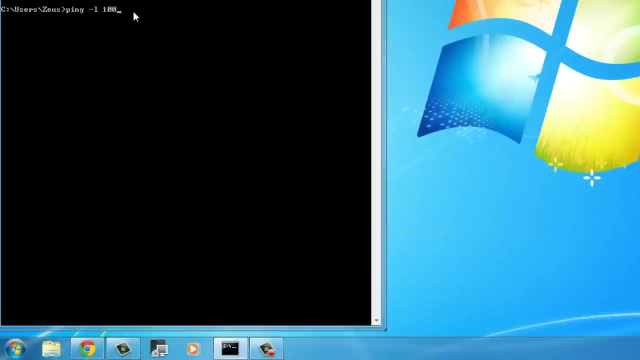 Or even 1000.. Okay, Let's do that again. We're bound to lose 13 packets. Okay to 100. and let's send this down to googlecom and remember, by default, it's going to send four packets. okay, we're not using the minus n parameter, we're using the minus l parameter, which allows me. 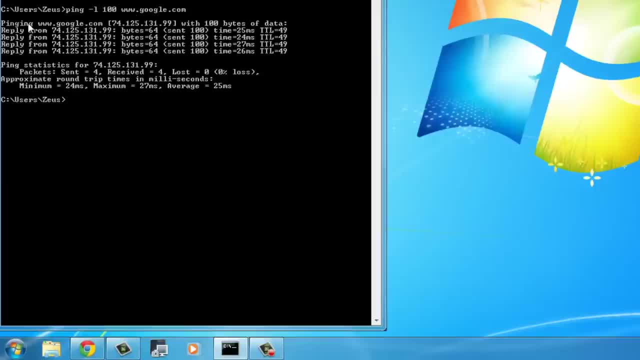 to designate the size. so if you look over here, it says pinging wwwgooglecom, google's ip address with 100 bytes of data. so i increased the size of the data and then again i sent four packets, i received four packets, i lost zero packets. so even with 100 bytes, the connection is pretty good. 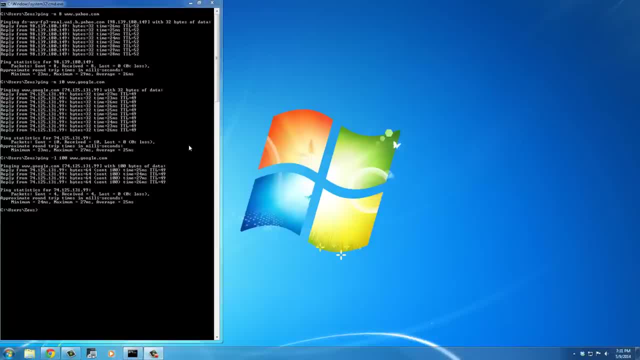 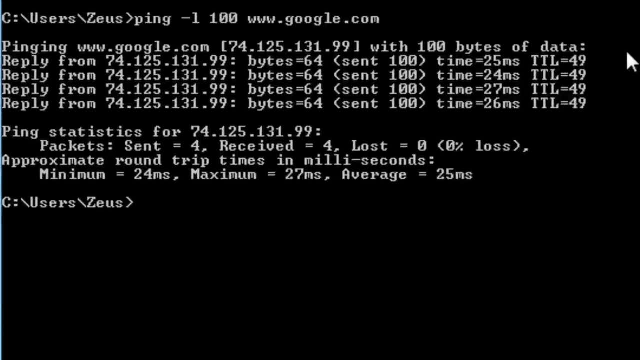 okay, i'm not losing any packets. okay. so there's one very important point i want to make before i move on. um, it pays off to analyze each line of data, okay? so here i pinged, google you with 100 bytes of packets. right, i sent 100 bytes, but if you look over here, i got a reply from: 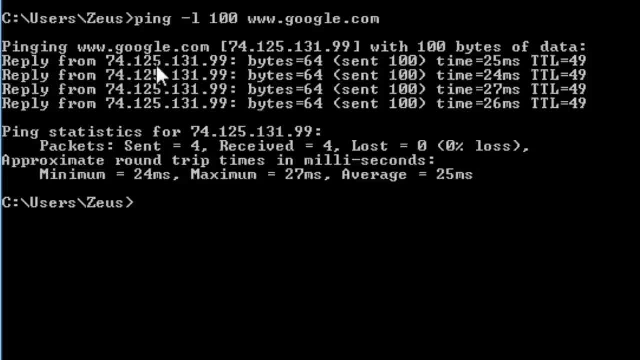 google- and this is google's ip address- 74.125.131.99, with a response of 64 bytes of data. so i sent 100 bytes, but google responded with a 64 byte packet. why? because i could have sent google one gigabytes, but google cannot respond with a. 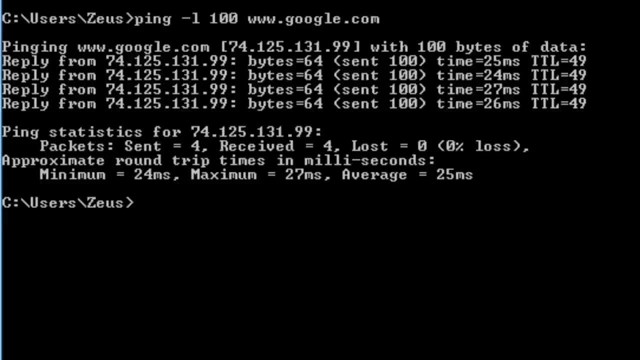 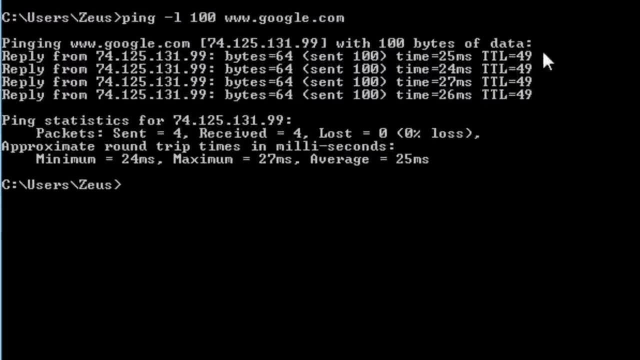 whole gig every single time. if they do that, their network connection will choke. so google probably have configured their servers to only respond with a maximum of 64 bytes to ping requests. okay, so i cannot send a ping request of one gigabytes to google. like i said, if i do that, their connections could choke. this could even be a form of an attack. i can sit. 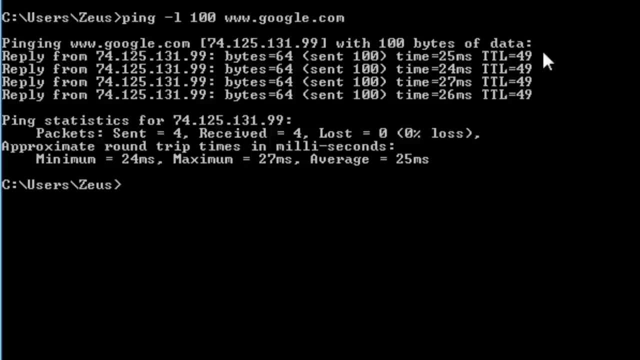 here and i can tell a hundred other people to keep pinging google all day with one gigabytes and that is going to choke google's servers. their connection speed is going to go down and people that are trying to access google are going to have problems. so even if i send 100 bytes of data, google only responds with the maximum of 64 bytes. 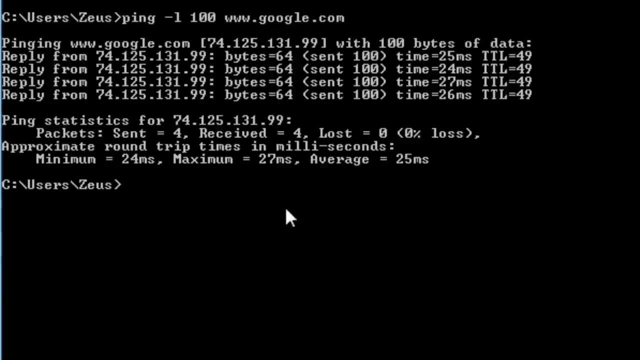 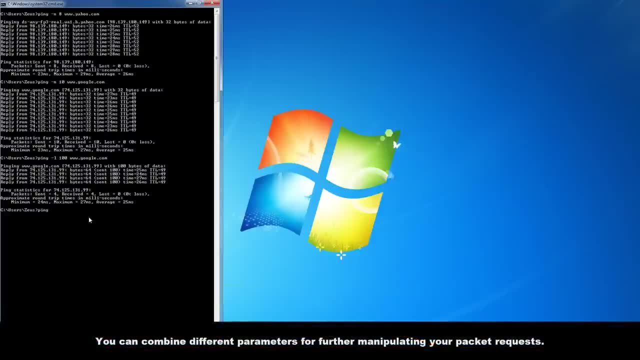 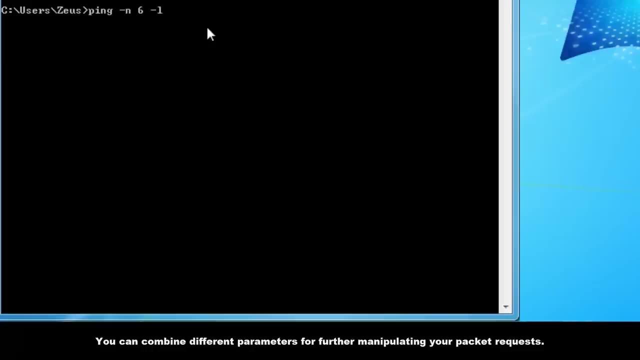 and 64 bytes is nothing, alrighty. and the final thing i'm going to go over with the ping command is how you can combine parameters so i can ping. let's say i'm going to ping google again. i'm going to ping google six times and i'm also going to send 64 bytes of data every single time. 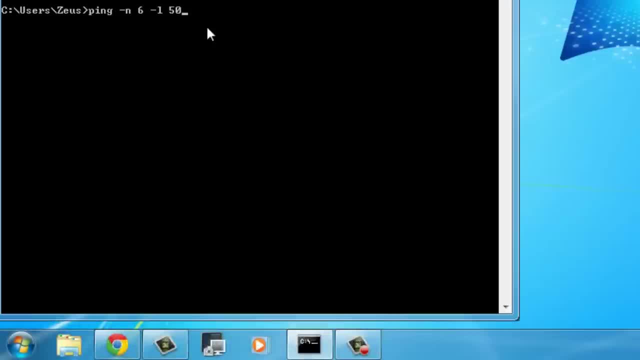 actually you know what. let's make that 50 bytes so i can actually combine parameters and use them together. dot com, so that's ping. minus n means ping x many times, so i'm going to ping it six times. and then minus l means designate the size of the data packet you're sending over, and that's going. 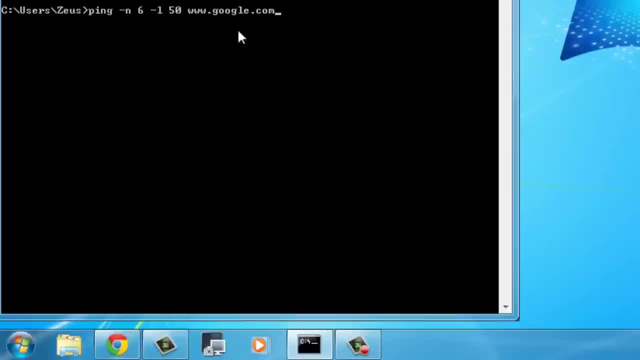 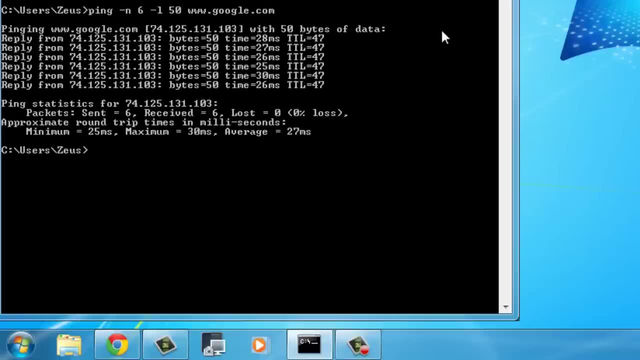 to be 50 bytes and i'm going to ping wwwgooglecom. press enter. let's wait for this to complete. okay, so we pinged google with 50 bytes of data. we pinged it six times: one, two, three, four, five, six- and google responded with 50 bytes of data. 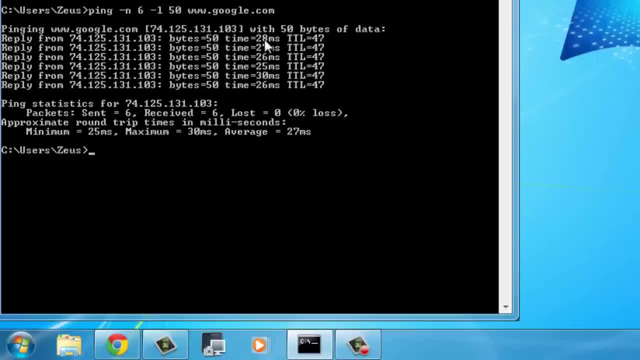 and they responded pretty quickly: 28 milliseconds the first time, 27 the next time, and the times varies a little bit. okay, but if you look at the bottom here, packet sent six, received six, lost, zero again. that means the connection is really, really good. but, as you can see, the point of this ping command was that you can combine the parameters. 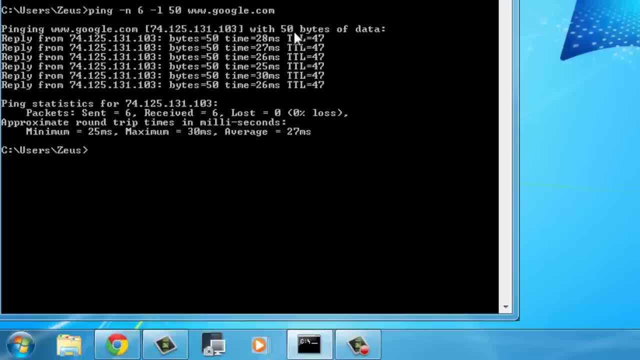 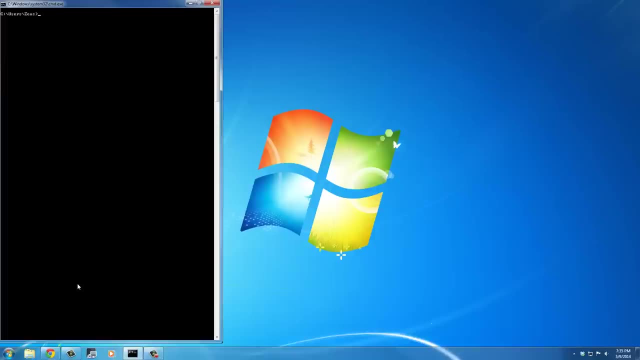 you can combine minus n with minus l to do two things at once. we were able to increase the size of packets we sent, the number of times we sent it over, all right, so let me clear the screen, cls, and then i'm going to show you one more thing, if you. 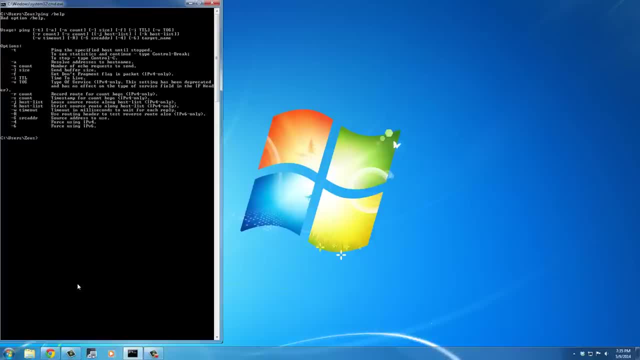 step in ping slash help. you will get a list of all the parameters that you can use and combine with each other over here. okay, i cannot show you all of them because some of them don't work, but uh, you can take a look at them if you're interested. but the minus n and minus l, i think, are the most. 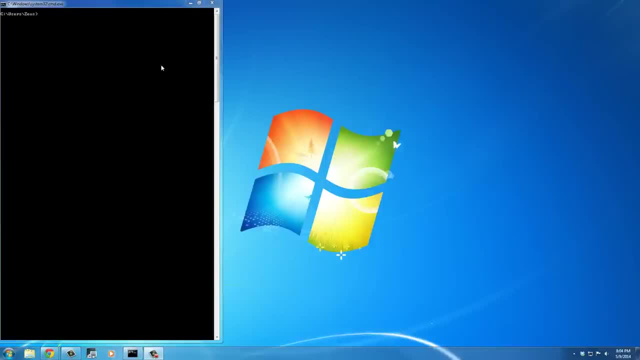 important. all right, so that's it about the ping command. so, basically, the ping command sends out an echo request and it gets an echo response if the device you're trying to reach is working- and this is how you troubleshoot your network- you have to make sure your router is.